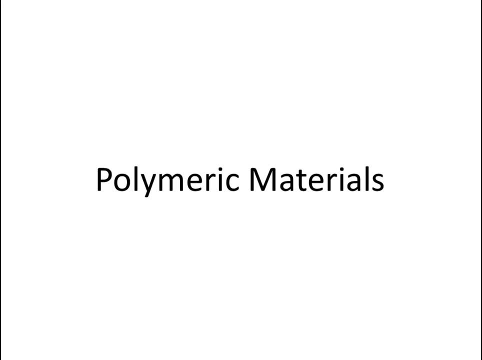 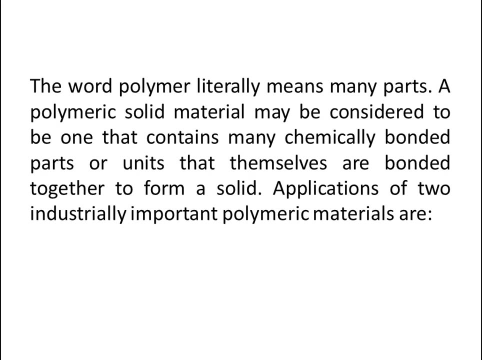 Hello everybody. Let's talk about polymeric materials Now let's begin. The word polymer literally means many parts. A polymeric solid material may be considered to be one that contains many chemically bonded parts or units that themselves are bonded together to form a solid. 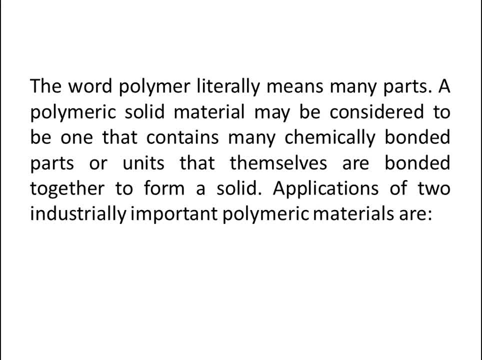 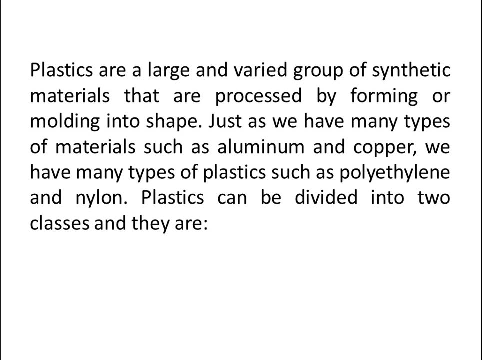 Application of two industrially important polymeric materials are plastic and elastomer. Plastics are a large and varied group of synthetic materials that are processed by forming or molding into shape. Just as we have many types of materials such as aluminium and copper, we have many types of plastics. 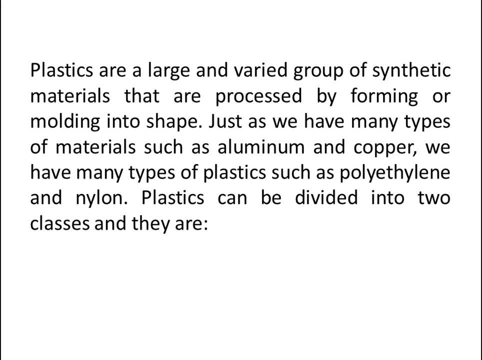 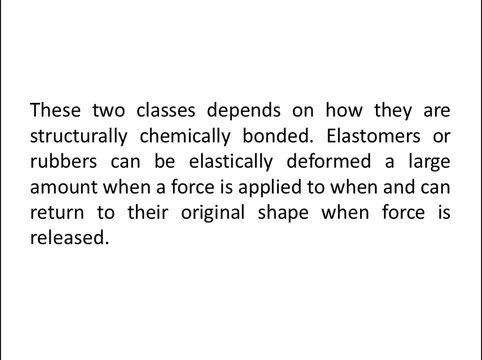 Such as polyethylene and nylon. Plastics can be divided into two classes and they are: first one is thermoplastics and second one is thermosetting plastics. These two classes depends on how they are structurally chemically bonded. Elastomers- rubbers can be elastically deformed a large amount when a force is applied to them. 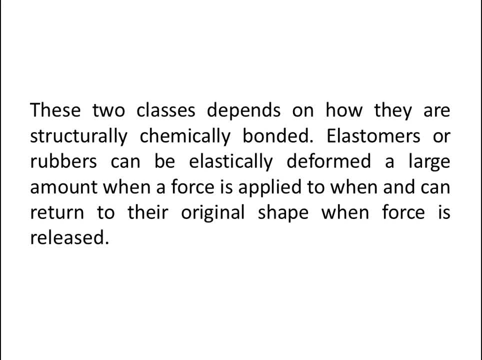 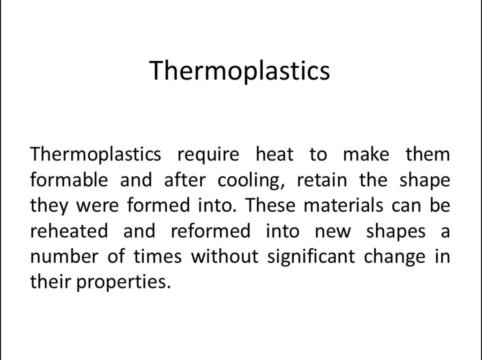 We are food to our brains, which can send it to the heart��자 when its original state gets formed. Let's talk about thermoplastics. Thermoplastics require heat to make them formable and, after cooling, retain shape. they are formed into And re-heating, restoration or smelting can be done with the help of Bath catching materials. 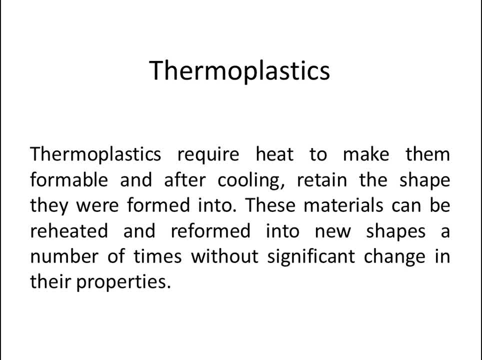 The materials can be reheated and reformed in new shapes a number of times without significant change in their properties. theoretically, wear it for a long time, leave some cracks on the extremely solid surface and dissolve fluid into waterounce. the material in the model can neverござint- has the ability to leave aseen tipsa. 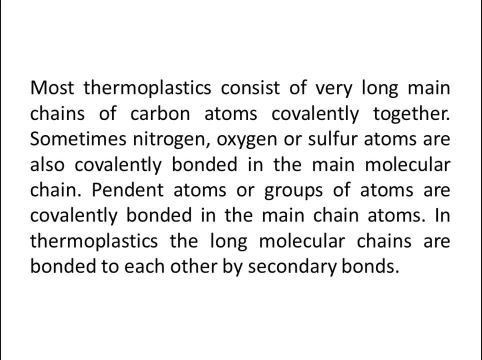 Most thermoplastics consist of very long main chains of carbon atoms covalently together. Sometimes nitrogen, oxygen or sulfur atoms are also covalently bonded in the main molecular chain. Pendant atoms or groups of atoms are covalently bonded in the main chain atoms. 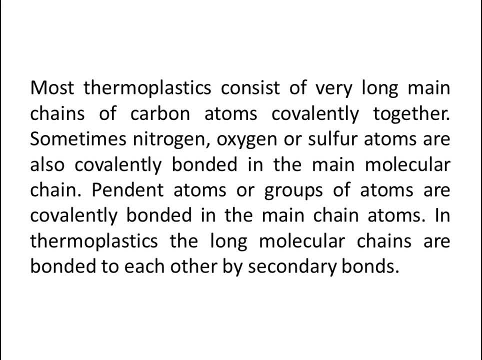 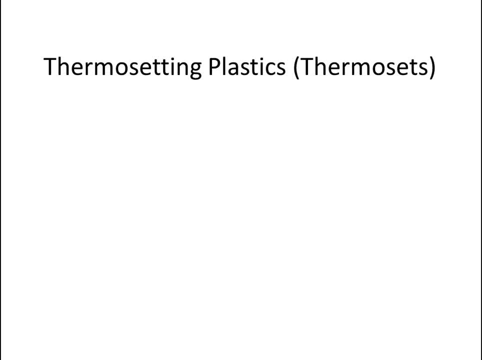 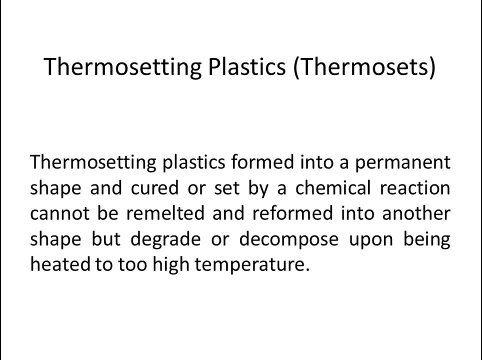 In thermoplastics, the long molecular chains are bonded to each other by secondary bonds. Now let's talk about thermosetting plastics or thermosets. Thermosetting plastics formed into a permanent shape and cured or set by a chemical reaction cannot be remelted and reformed into another shape. 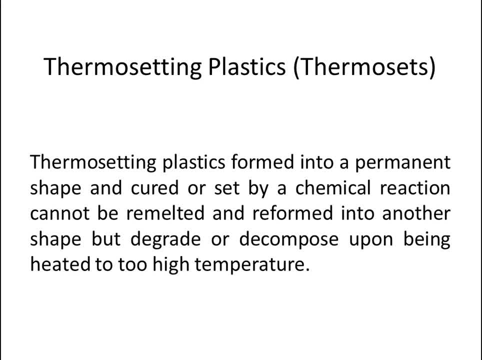 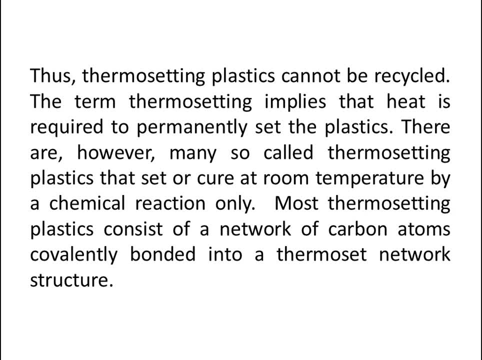 but degrade or re-melt or decompose upon being heated to too high temperature. Thus, thermosetting plastics cannot be recycled. The term thermosetting implies that heat is required to permanently set the plastics. There are, however, many so-called thermosetting plastics that set or cure at room temperature. 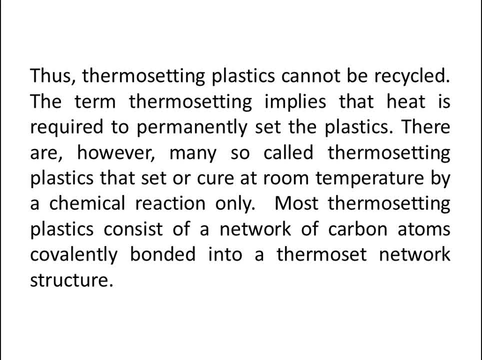 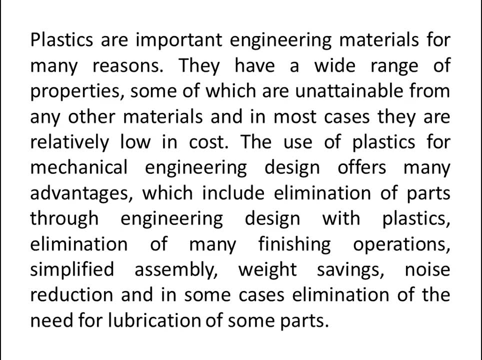 by a chemical reaction only. Most thermosetting plastics consist of a permanent shape or set by a chemical reaction. The thermosetting plastics consist of a network of carbon atoms covalently bonded into a thermoset network structure. Plastics are important engineering materials for many reasons. 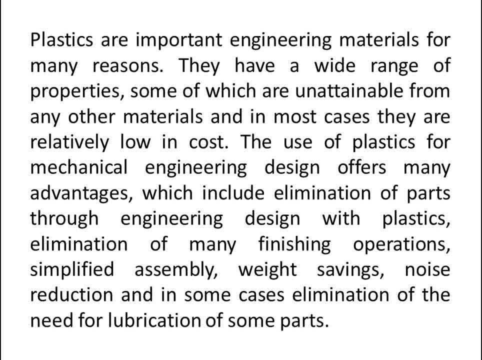 They have a wide range of properties, some of which are unattainable from any other materials, and in most cases they are relatively low in cost. The use of plastics for mechanical engineering design offers many advantages. The use of plastics for mechanical engineering design offers many advantages. 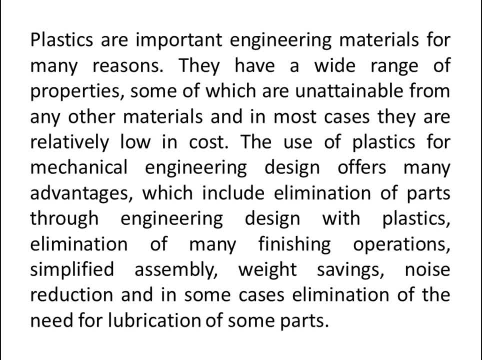 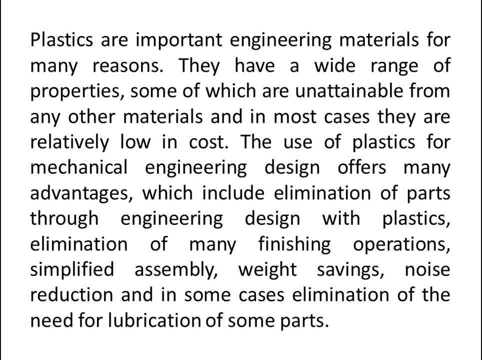 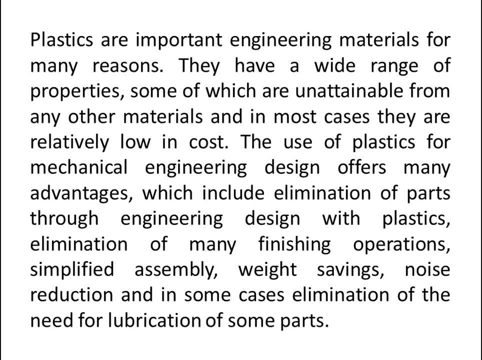 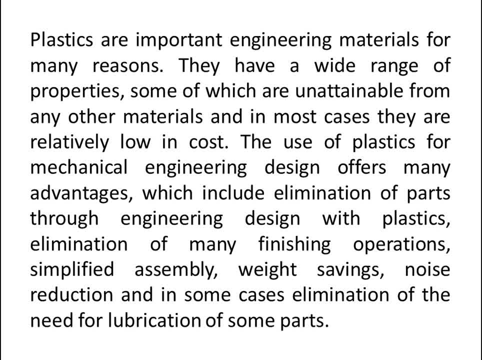 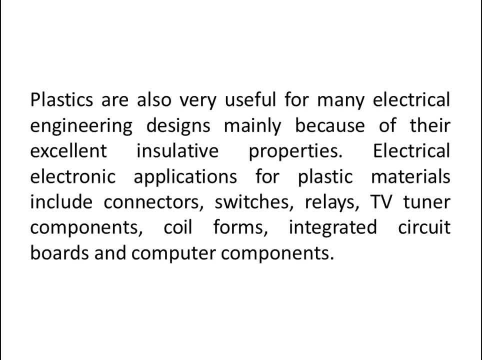 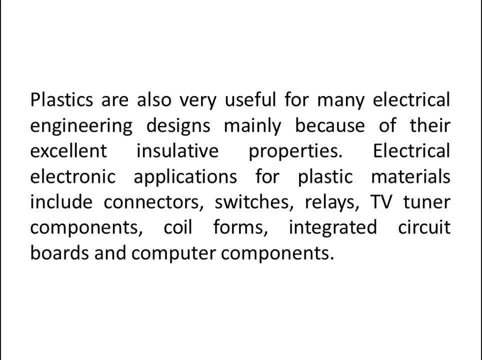 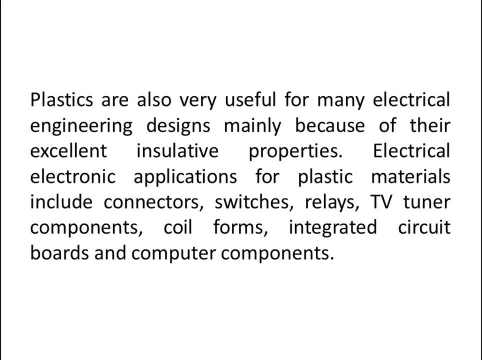 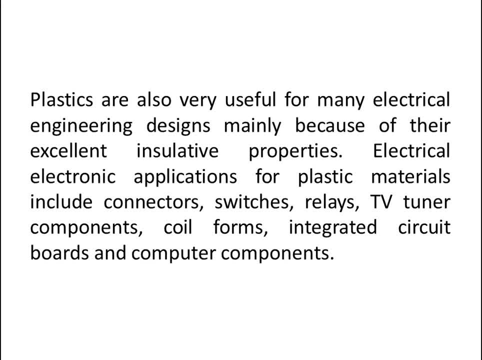 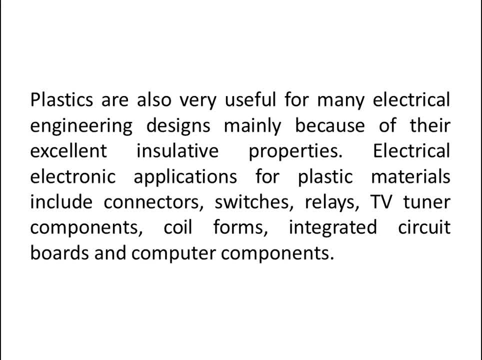 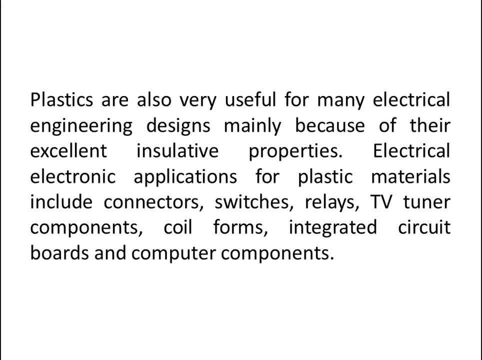 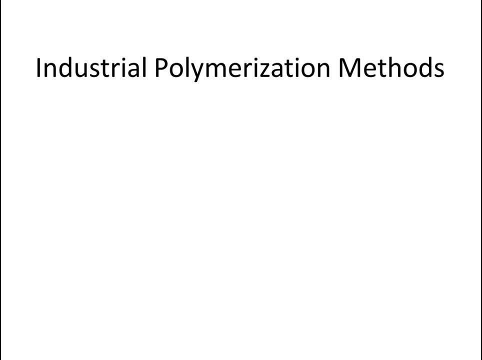 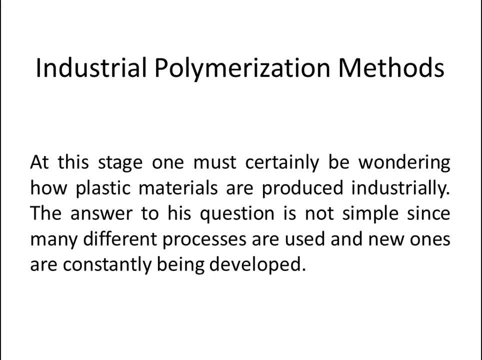 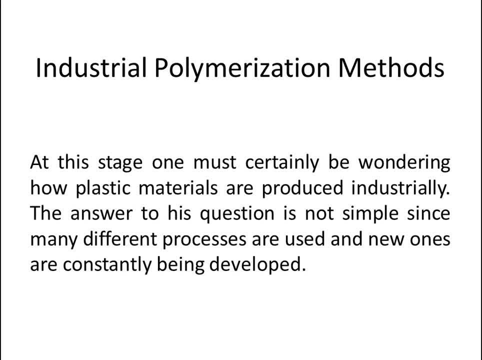 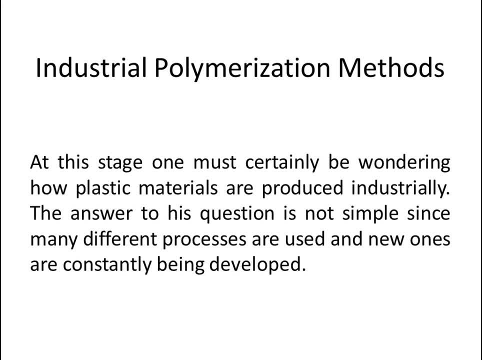 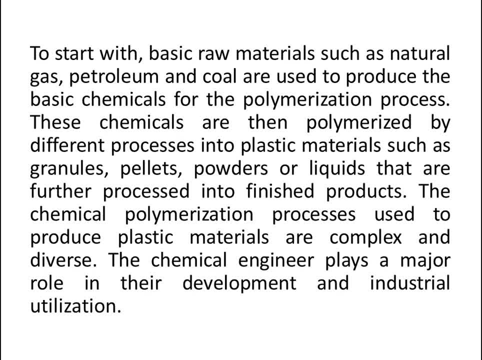 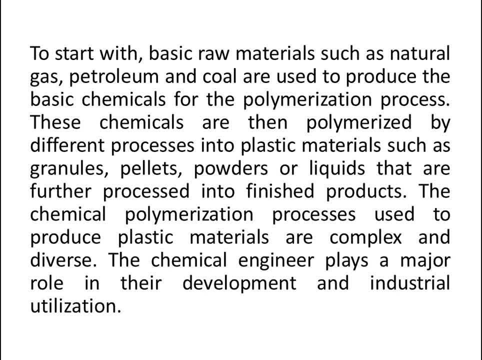 The use of plastics for mechanical engineering design offers many advantages. Plastic chrome materials such as natural gas, petroleum and coal are used to produce the basic chemicals for the polymerization process. These chemicals are then polymerized by different processes into plastic materials such as granules. 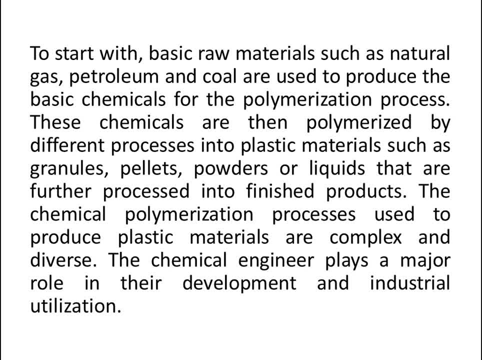 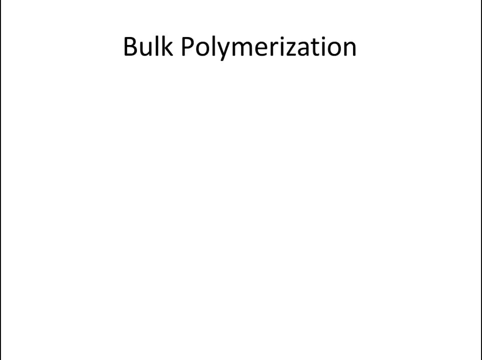 pellets, powders or liquids that are further processed into finished products. The chemical polymerization processes used to produce plastic materials that are complex and diverse. The chemical engineer plays a major role in the development and industrial utilization. Now let's talk about bulk polymerization. 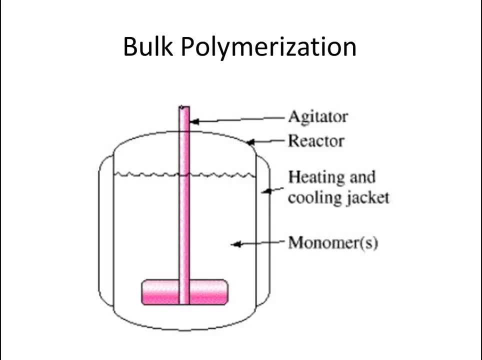 There is a figure for this one, and here we can see: this one is the agitator and this is the reactor for making the plastic. and this one is this, and this one are the heating units, This is the heating and cooling jacket, and here there are monomers. 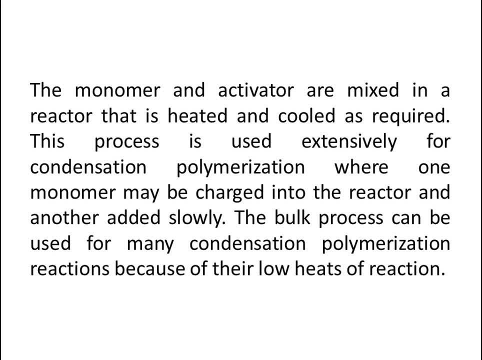 The monomer and activator are mixed in a reactor that is heated and cooled as required. in this system. This process is used extensively for condensation polymerization, where one monomer may be charged into the reactor and another added slowly. The bulk process can be used for many condensation polymerization reactions. 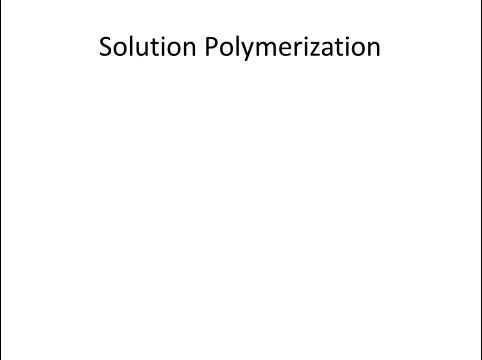 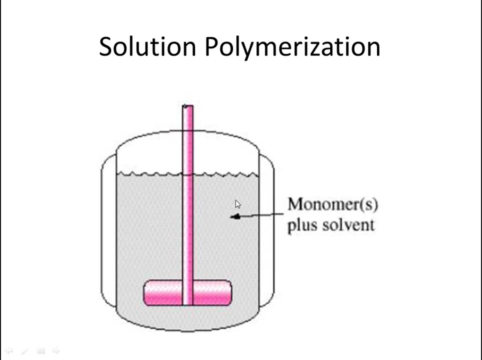 The bulk process may require a cadaver of a collected heat of a particular reactor. Now let's talk about solid polymerization. Now, the figure is here And the other things are exactly the previous one, and here there are monomers and as well as solvent. 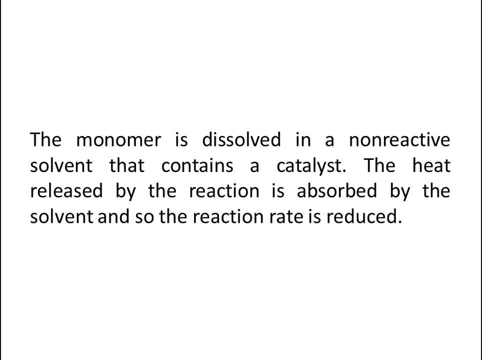 Now, in this process, the monomer is dissolved into a non-reactive solvent that contains a catalyst. The heat released by the reaction is as little as a liter of heat is absorbed by the solvent end, so the reaction rate is reduced. now let's talk about suspension. 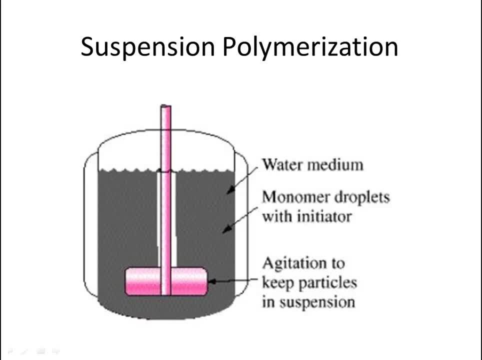 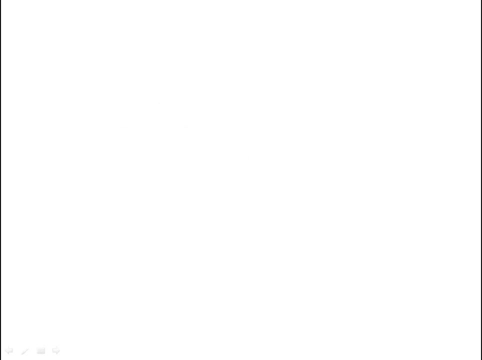 polymerization and there is a picture for this one and this, this one and this one is also the similar, like the previous one, and here there is water medium and also there is monomer droplets with initiator and there is a theater, the function of alligator to keep particles in suspension in 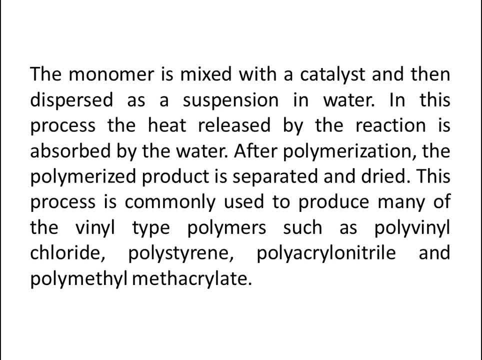 this process, the monomer is mixed with a catalyst and then this passed as a suspension in water. in this process, the heat released by the reaction is absorbed by the water. after polymerization, the polymerized product is separated and right. this process is commonly used to To produce many of the vinyl type polymers, such as polyvinyl chloride, polystyrene, polyacrylonitrylate and polymethylmethylcrylate. 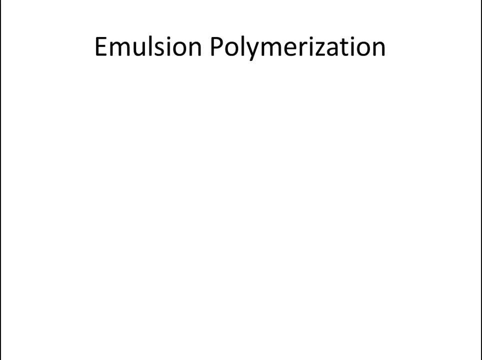 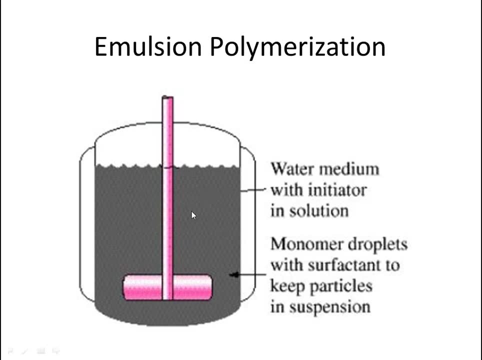 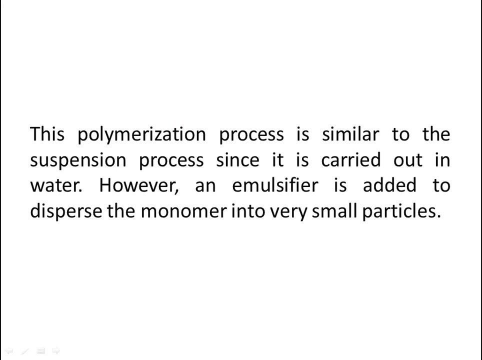 Now let's talk about emulsion, polymerization, and there is a figure for this one, and here we have a water medium with initiator in solution and there is also monomer droplets with surfactant to keep particles in suspension. And in this process, the polymerization process is similar to the suspension process, since it is carried out in water. 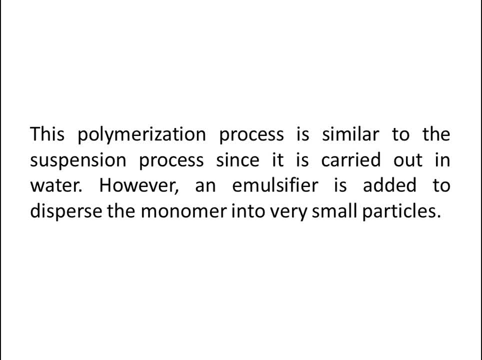 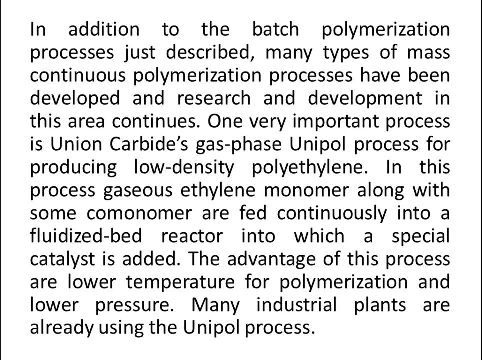 However, an emulsifier is added to disperse the monomer into very small particles. In addition to the batch polymerization process just described, many types of mass continuous polymerization process have been developed and research and development in this area continues. One very important process is unial carbide gas phase unipole process. 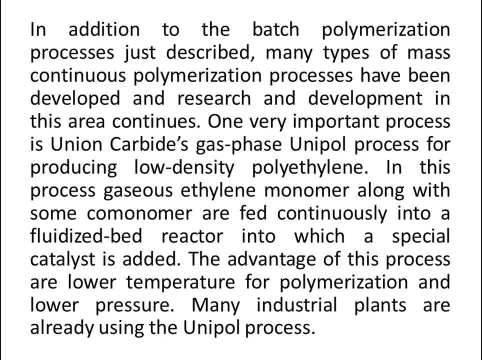 For producing low density polyethylene. in this process, gaseous ethylene monomer along with some common monomer are fed continuously into a fluidized bed based reactor into which a special catalyst is added. The advantage of this process are lower temperature for polymerization and lower pressure. 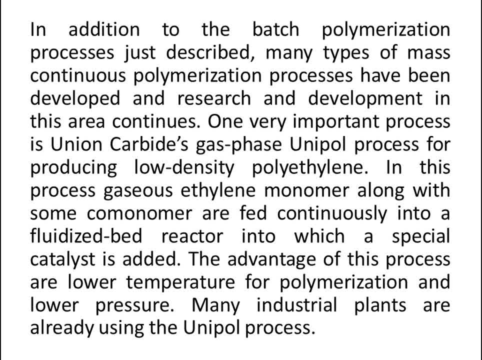 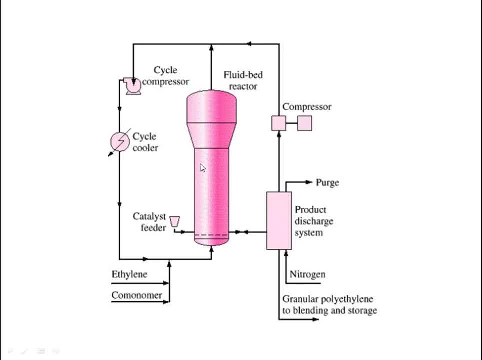 Many industrial plants are already using the unipole process And there is a schematic diagram for this one. So the center, there is fluid bed reactor and the fluid bed reactor. fluid goes to cycle compressor and from cycle compressor the fluid goes to cycle cooler. 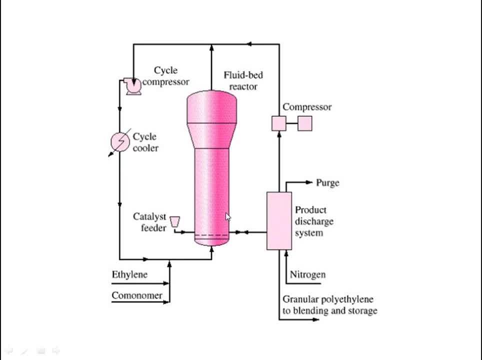 Then from cycle cooler the fluid again go to the fluid bed reactor and here ethylene and some common monomer is added And also catalyst is added here. And from this fluid weight reactor the fluid goes to product discharge system. Also from product discharge system the fluid goes to the fluid weight reactor And the product from the product discharge system goes to purge. Also goes to granular polyethylene for blending and storage.